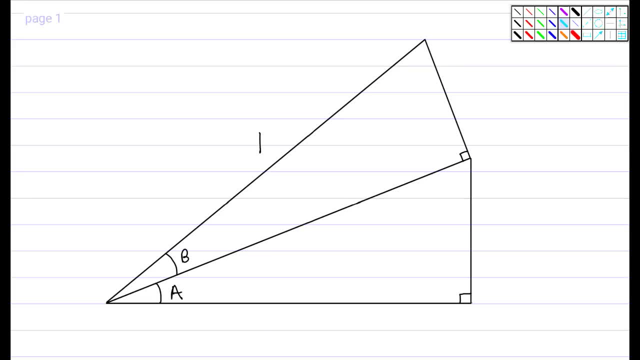 Hello mathy people out there. Today we're going to be proving what are called the addition formulas for sine and cosine. So specifically, we want to learn what is sine of a plus b and what is cosine of a plus b in terms of the sines and cosines of these angles separately. 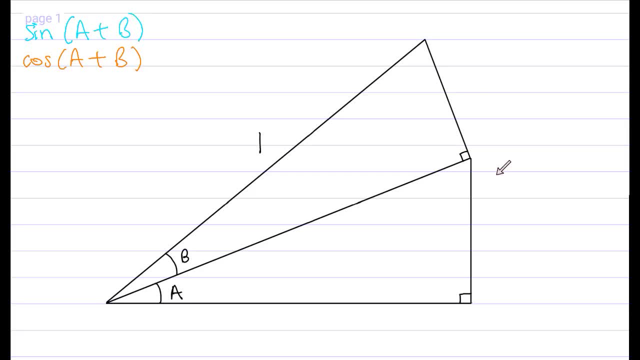 And using this diagram, we can prove that. Okay, here I've got a nice right triangle, and on top of that I've got another right triangle. The first triangle has an angle a down here, the second triangle has an angle of b and the second triangle also has a hypotenuse of one. Okay now, before we 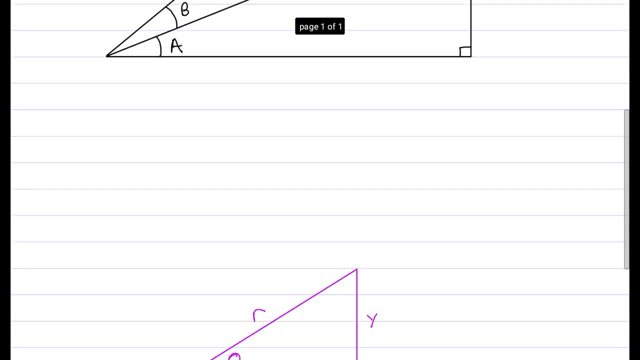 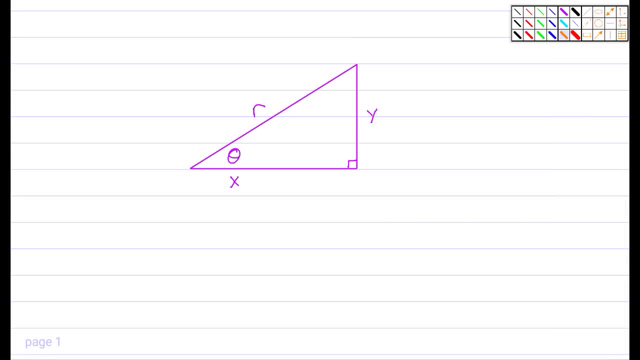 start with that. let's just get a little refresher on. you know what the definitions of sine and cosine are. Let's just get a little refresher on what the definitions of sine and cosine are Really quick. we're going to need this when we do this proof. Remember that cosine of theta. 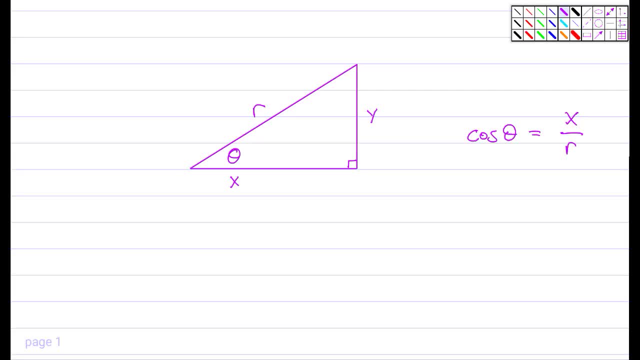 right is defined as x over r. for a triangle like this, Sine of theta is defined as y over r. So if I just solve these two equations for x and y, I can figure out what my legs are. y is equal to r sine theta. x is去了 from r to theta. So I just solve these two equations for x and y, I can figure out what my legs are. Y is equal to r sine theta x is squarer than theta and x is equal to y. 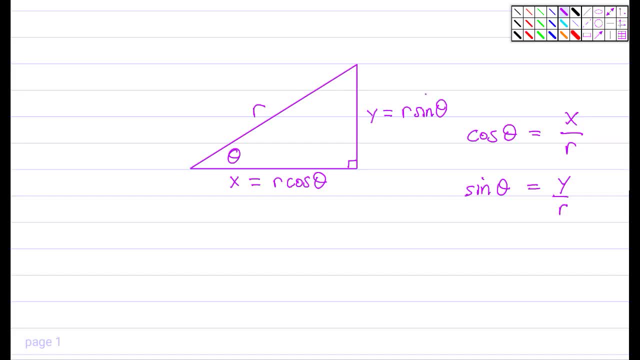 equal to r cosine theta. This is useful if we know the angle and we know the hypotenuse. then this gives us the other two sides of the triangle. It's got to be a right triangle, but the other two sides of the triangle right away. So we're 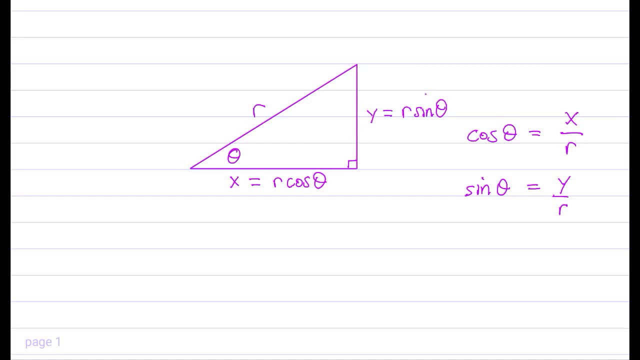 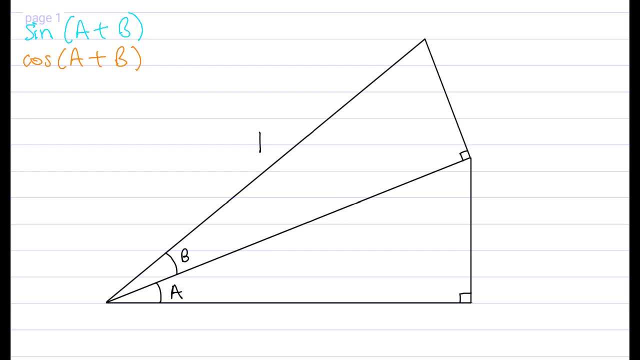 going to need this when we do our proof. Okay, so let's start. Well, if I know that the side of this triangle up here, the hypotenuse of this upper triangle is 1, and I know this angle is B, I know that. 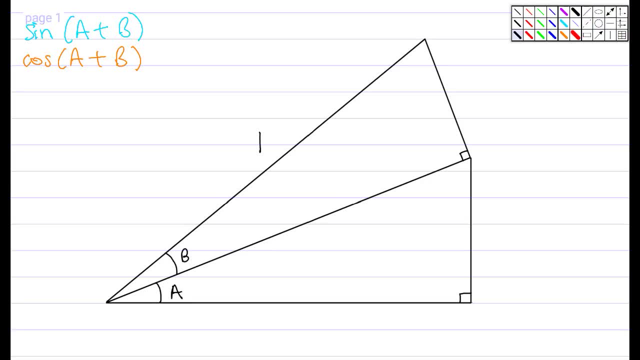 this side up here, this leg on the top triangle is sine of B and I know that this other leg, this long leg down here, is cosine of B. Well, if I know that the hypotenuse of the lower triangle is sine of B, then I know that this side up here, 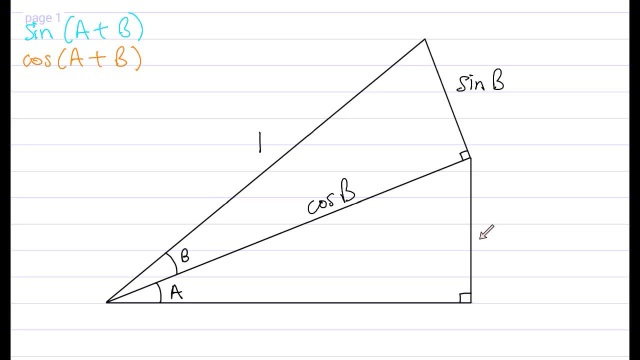 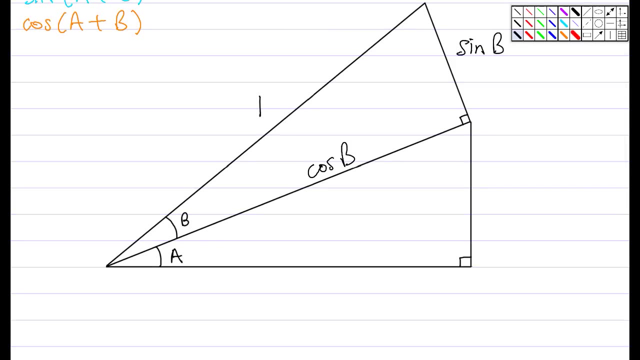 is cosine of B, then I can figure out the other two legs right, basically doing what we just went over, which is take the hypotenuse multiply by sine of this angle right here, and that's this side, Cosine of B, sine of the angle. Similarly, 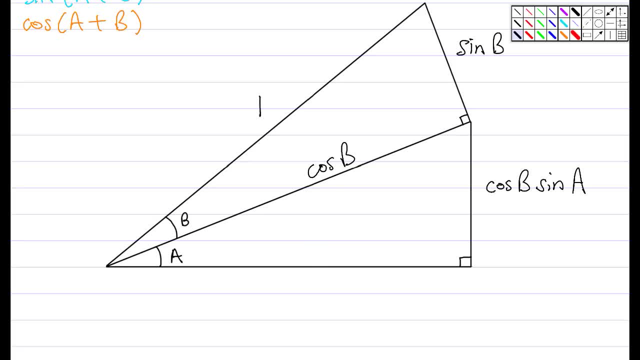 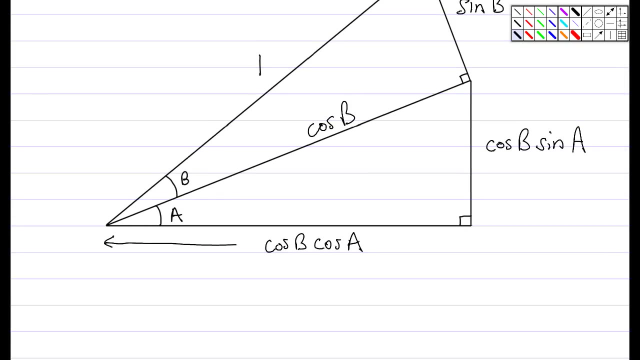 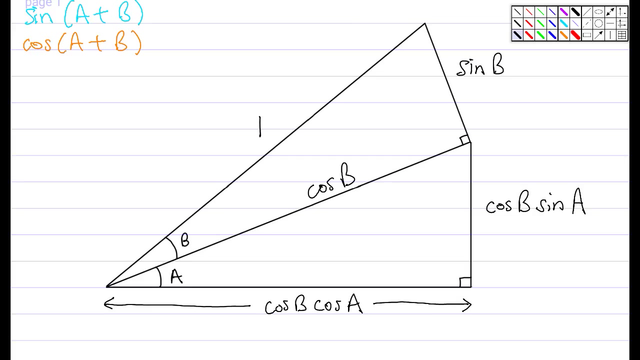 this leg down here is cosine of B times, the cosine of the angle, And that is this entire, that's this entire thing right here. There we go. Okay, I'm hoping you're with me so far. We have to make this diagram a. 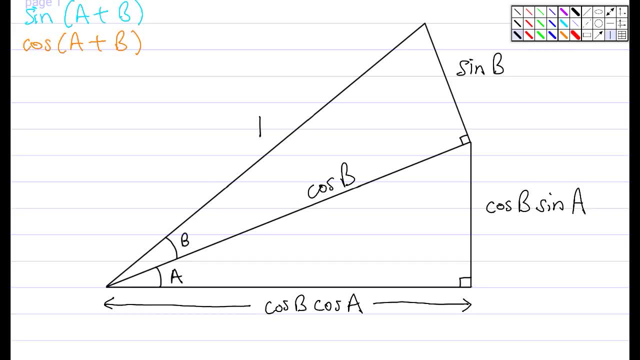 little bit more complicated, but it's not too bad. Okay, I'm hoping you're with me so far. We have to make this diagram a little bit more complicated, but it's not too bad. So just follow what I'm doing. I'm going to take a straight line and go. 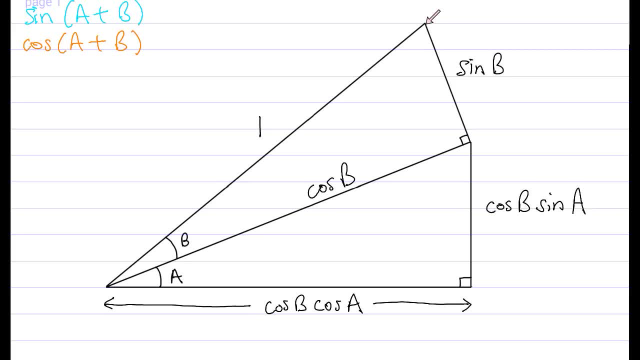 straight down from this point very top there. Okay, nice vertical line, It's going to reach the bottom here at a nice right angle. I'll draw in a little right angle symbol And then one more line and there won't be any more lines, I promise. Go draw. 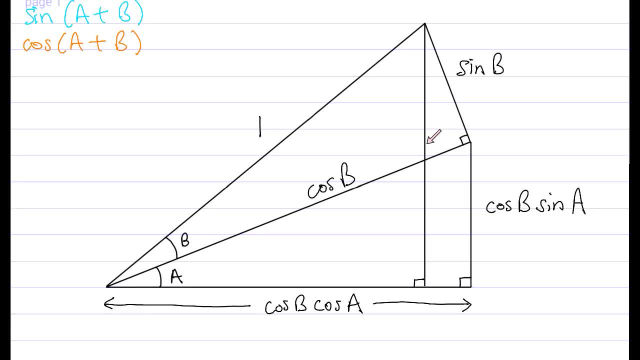 a line right here which meets this line and at a right angle and intersects at this vertex point right here. There we go nice horizontal line Right from that point. It's a little bit small, Hopefully you can see it. 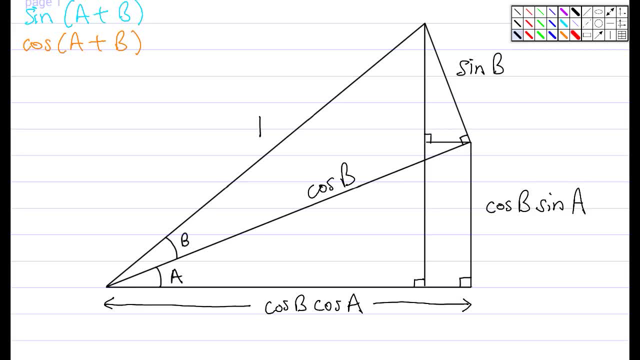 I'll put in the right angle so we know that's also a right triangle. Okay, well, notice this angle A and notice that this little segment here is parallel to this little segment here, And notice that this little segment here is parallel to this little segment. 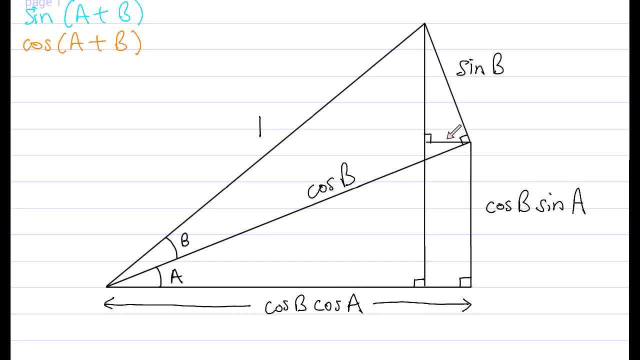 here And notice that this little segment here is parallel to this little segment here. This big segment here is parallel to this little segment right here And this angle is A. well, we have an alternate interior angle right here. You can see where my arrow. 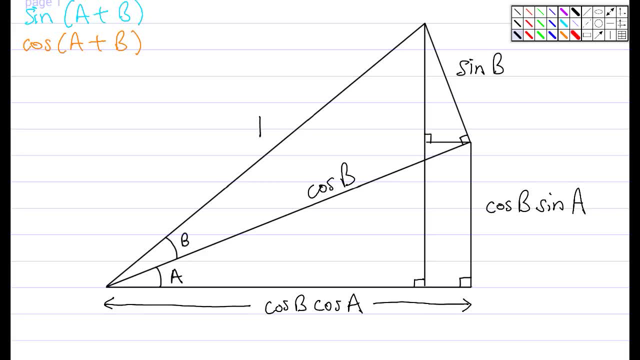 is That angle is also A, so I'll just label that as A. If this angle is A and this full angle is 90 degrees, then this angle must be 90 minus A, And then, if you look at this triangle right here, this is 90,, this is 90 minus A. We now 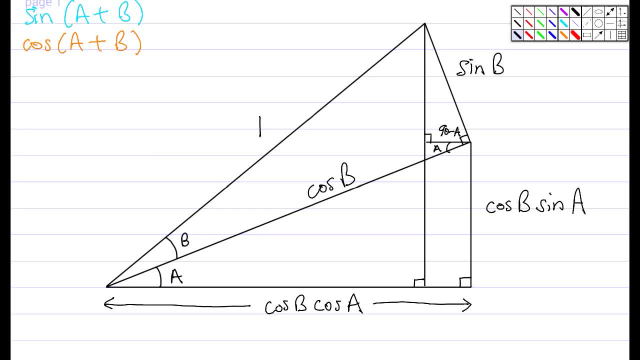 know that this angle is up here. That angle is also A. Okay, so it turns out this angle up here is the same as this angle down here, So let's focus on this triangle right now. It's got a hypotenuse sine B and my angle. 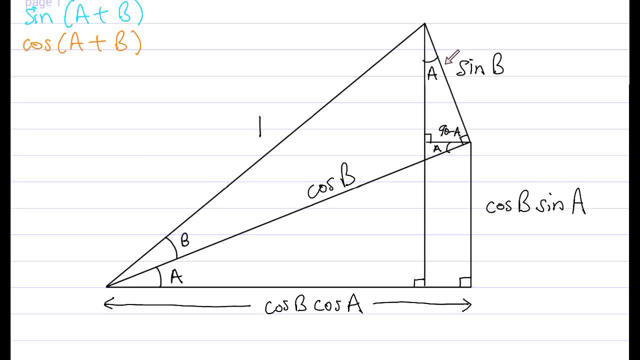 is A. We're using the same trick that we've been using before to get like this side and this side and this side. Here's the hypotenuse, here's the angle. this is the adjacent side. So I know that this side is sine of B, cosine of A. That's this side, from here right to. 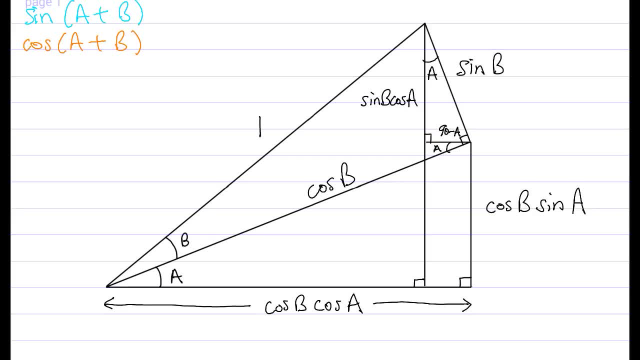 here. Well, we also know what the length of this line segment is. That one's a tough one to label. I'm just going to put it here. I'm just going to put it here. I'm just going to put it over here. 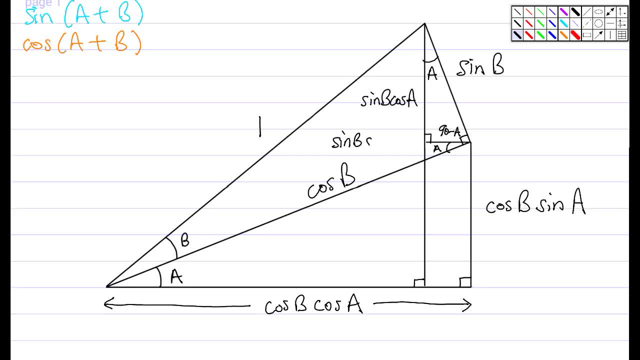 That's the hypotenuse times, the sine of the angle. I'll draw a little arrow there so we know what that is. There we go. That was the length of this, right here. Sine B, sine A is the length of this. 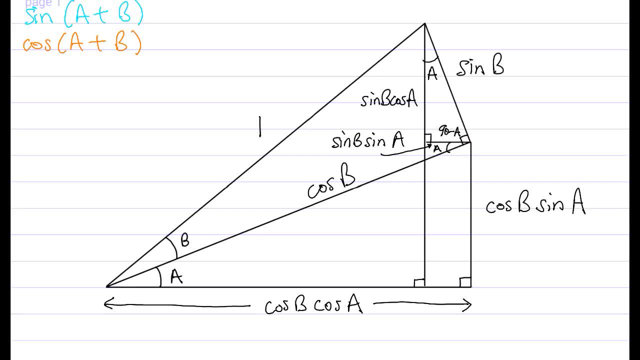 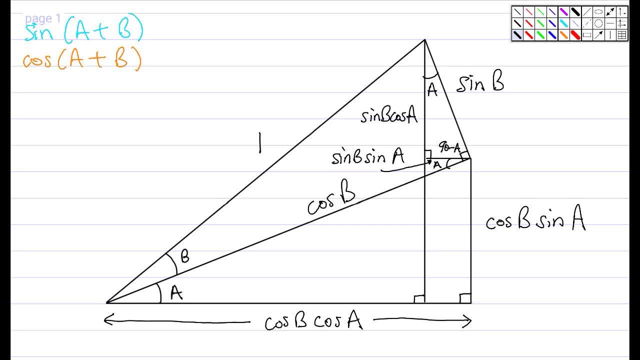 side. Well, we're actually just about ready to give our proof. We're basically done, Okay, Okay. One thing to notice is that what is the length of this big segment right here? Well, if you see this triangle right here's the three sides, right like that. It has a hypotenuse.